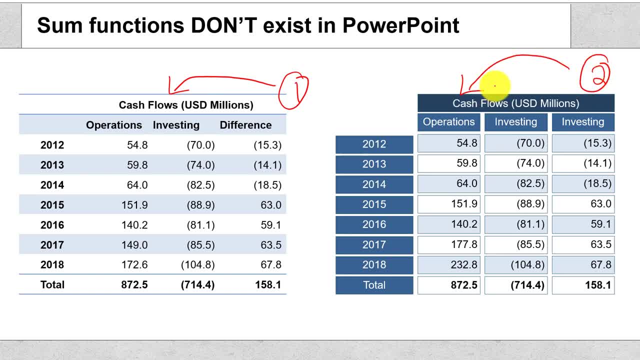 have that same table of cash flows built out using rectangles here in PowerPoint. The issue is all of these totals down below both over here from my graphic and my table are incorrect because I've actually deleted out two of the rows that used to be here but I never came. 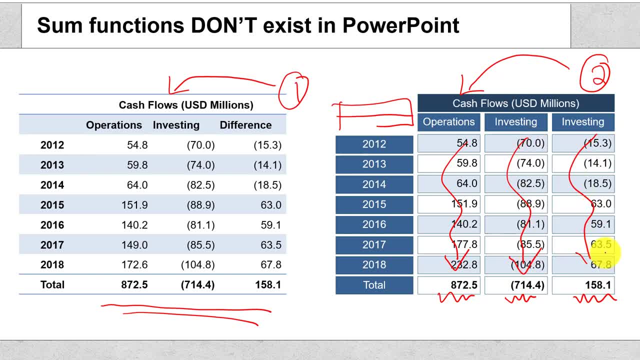 and updated these different totals. So this is why you can never trust totals in PowerPoint. There is no such thing. I repeat, there is no such thing as a sum function here in PowerPoint, even if you're using a PowerPoint table. If I come into PowerPoint, I can prove that to. 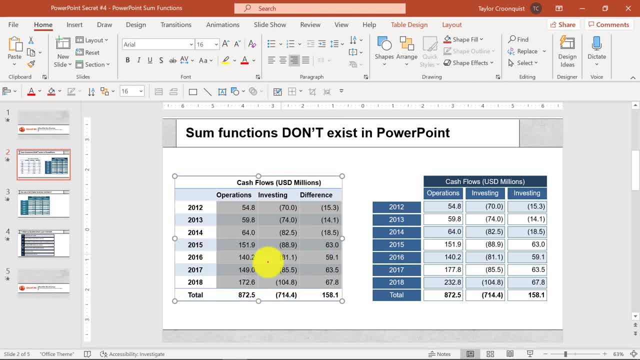 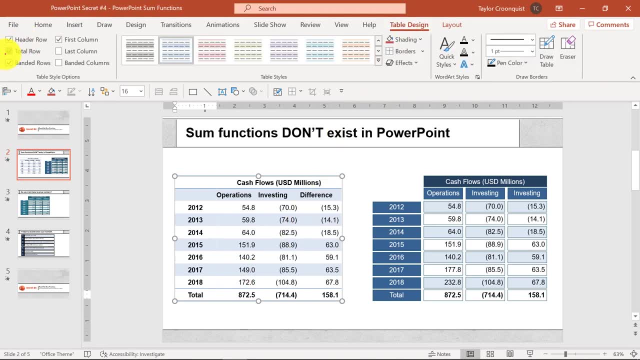 you. So here I have a table which is going to behave totally different than a table in Excel. Here it looks like I have this total row and if you come to the table design tab, this is often mistaken as a sum function, total row, which it's not Notice as I turn it on. 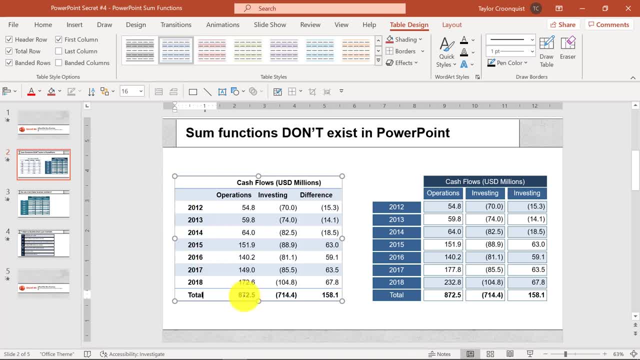 and off. I'm just getting different formatting down below. So all of these numbers are manually typed in or copy and pasted from Excel. If you have a table like this, you can just copy and paste them into Excel. but what do you do if someone's built a graphic like this? 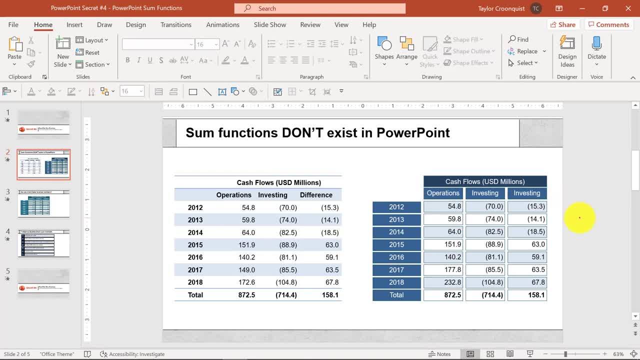 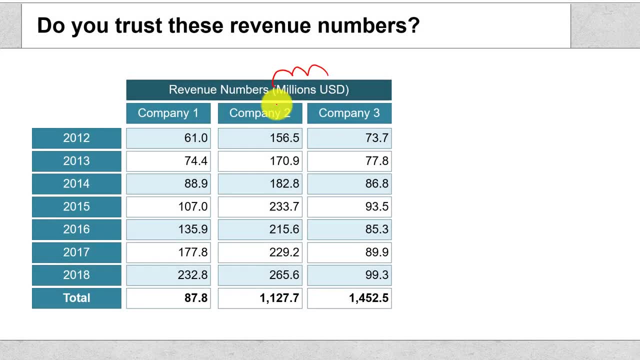 So here I have just a bunch of rectangles with numbers in them. How do you double check this? And if I come to the next slide, here is a classic example of something like this. So would you trust these millions USD revenue numbers for these three companies And hopefully, 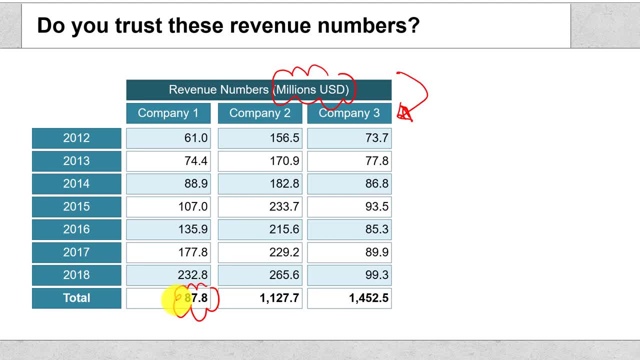 your answer is no, Right off the bat. you can see that this total is actually less than the numbers it's actually adding up. If you kind of eyeball this on the right, I have seven columns, all of them which are less than a hundred million in revenue, which means 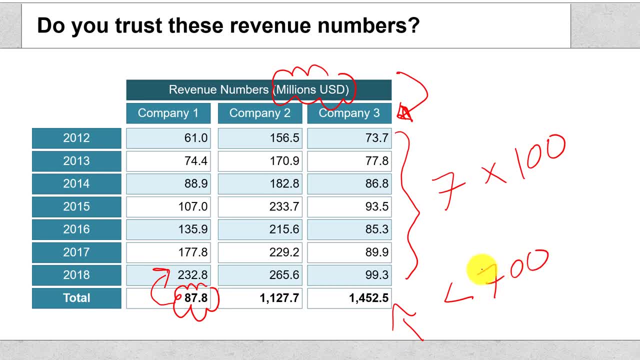 that this total has to be south of 700 million in revenue, which obviously brings up the question: is this total correct? which of course it's not, because I deleted some rows and messed up some of the numbers. now, how would you do this? a lot of people would just start to copy and paste these numbers into 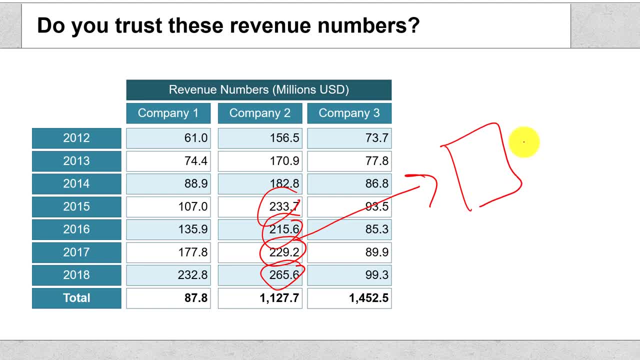 excel. you might even break out your iphone or smartphone calculator to try to come up with these numbers. but imagine if you had 10, 20, 30 or even 50 graphics like this in a deck and you needed to make sure that all these numbers were correct super, super fast. so that's what today's insider 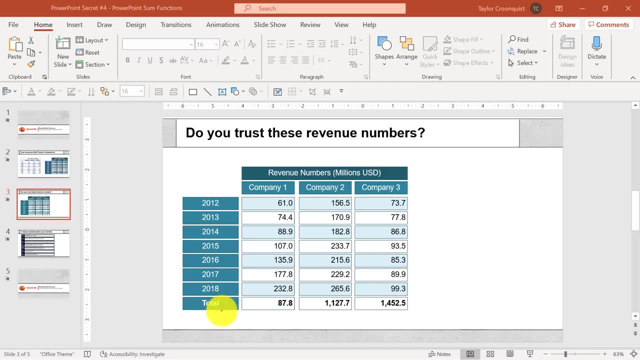 secrets going to show you how to do to do that. simply come into powerpoint and the first thing you're going to want to do- we are going to totally trash this graphic using these tricks. so the first thing you're going to want to do is hit ctrl shift d on your keyboard to create a duplicate. all right, 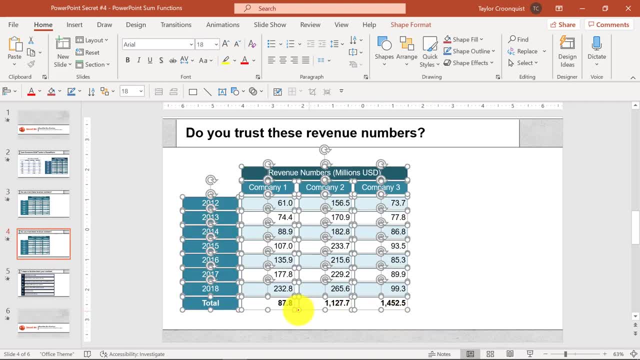 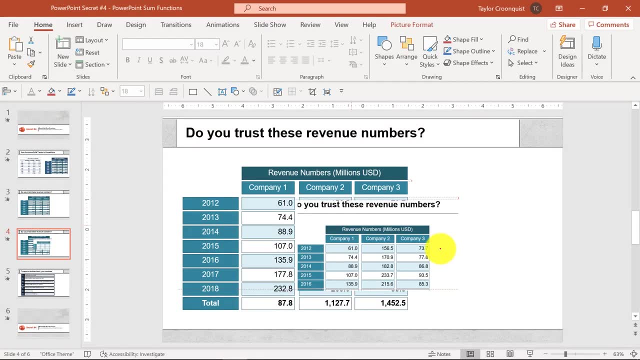 of your slide. so this is the slide that we're totally going to trash to get to the correct totals. the next thing you want to do is add a picture. i'm just going to hit windows shift s i'll quickly screen snip and control v to paste a copy of my slide as a picture, and this picture is going to. 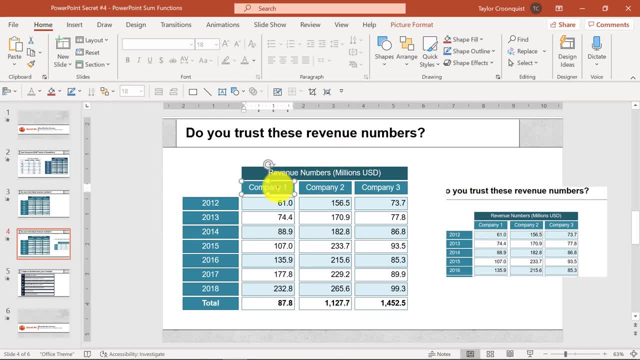 get lost, so you don't have to worry about what this looks like now. the next thing you need to do is select the numbers in the order you want them. so if you select your numbers vertically, one by one, they will stack up vertically. if you select them horizontally, they're going to stack up horizontally. in this case, i do want my company. 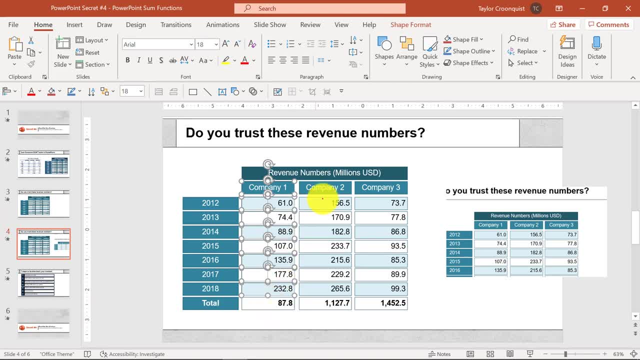 one numbers, so you're going to quickly click through these. i'm not going to click the total because i know it's incorrect. i'm then going to holding shift, click my company- two numbers. then i'm going to hold and shift, select my company- three numbers, and i recommend doing them. 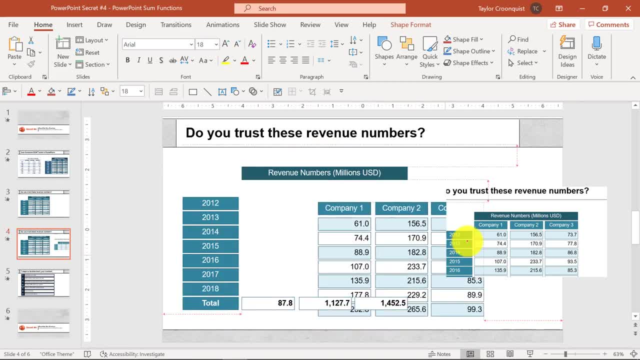 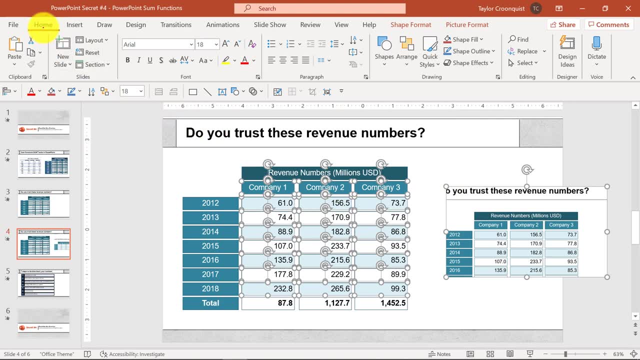 one by one like this, so you make sure you get all the numbers. i'm going to move them around. you can see i have all of my numbers holding shift. you then want to select your picture so that we can push this through smarter. now, right off the bat, if you come to the home tab, notice. 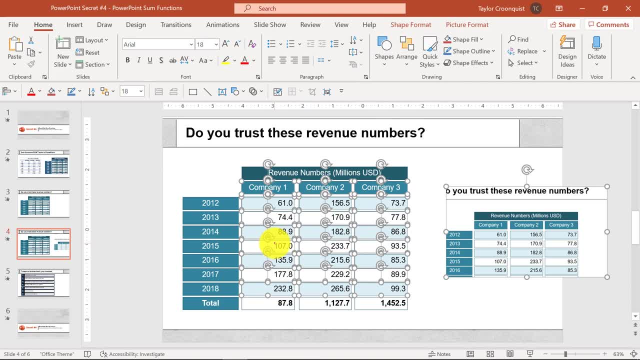 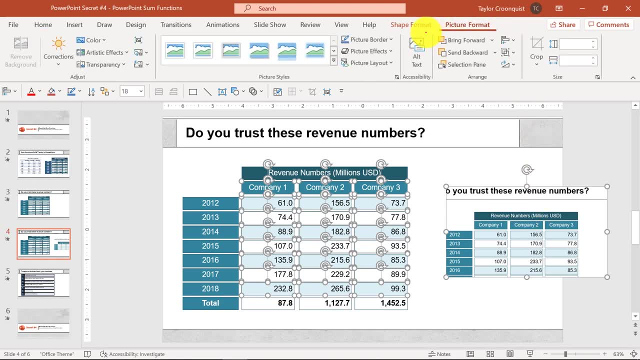 that the smart drop down is grayed out, so you cannot push rectangles as they are from the home tab into smart art. but because we now selected this picture, you can picture, format, picture layout and you can just pop these into a graphic. now all of these are going to look: 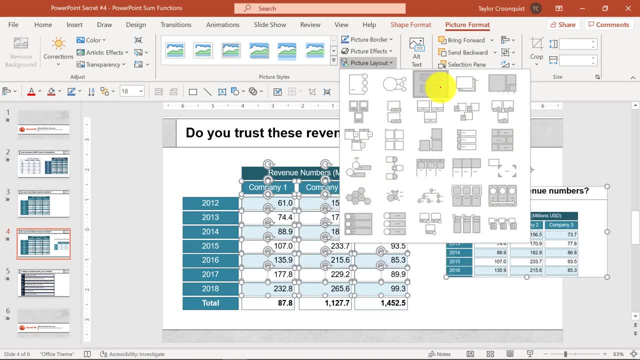 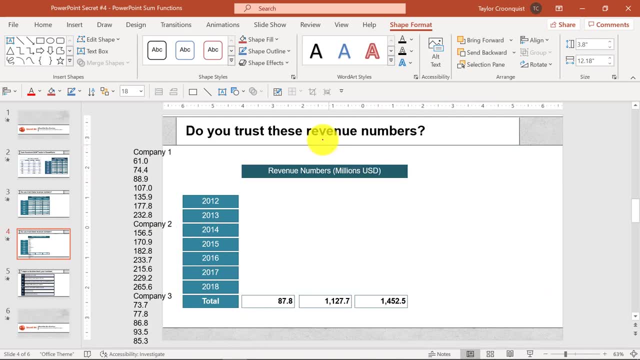 completely ridiculous. it doesn't matter which one you pick. you're going to select your graphic, it's going to tear your gra, your graphic, apart, convert to convert to text and kaboom, there are all of your numbers from the shapes now in a single text box that i'll 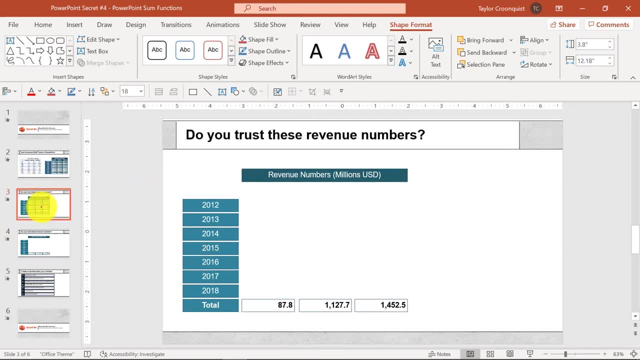 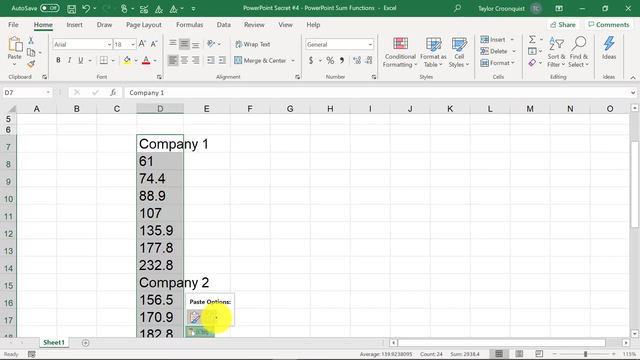 show you how to do that in just a second. i'm going to go over to excel and i'm going to go over to control a to select all. control x to cut them. we'll come back to the slide that we're going to double check the numbers on. i'm going to go over to excel. i'm going to control v to paste. 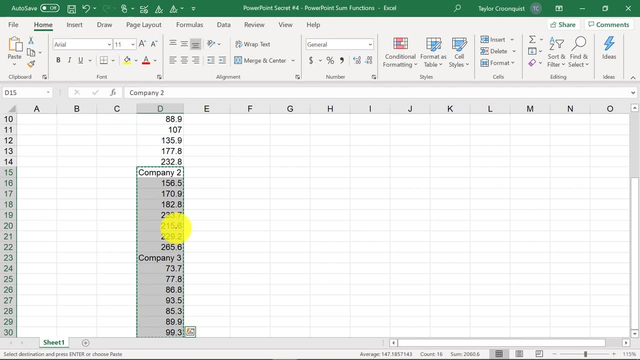 them in. i'm going to paste as text so that it converts to control b to bold. i don't want everything bold. i'm going to copy that line of text. i'm going to copy the next line of text, which will x, and from here, now that i have them in these columns, i can simply.